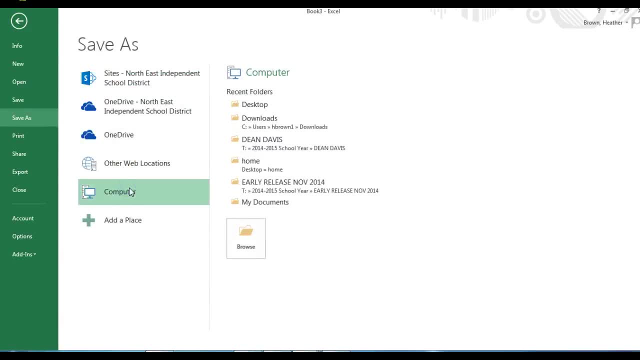 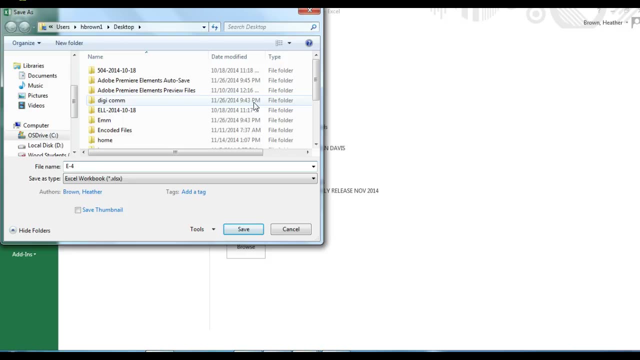 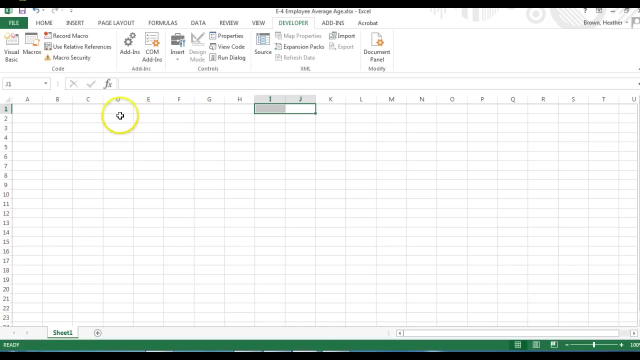 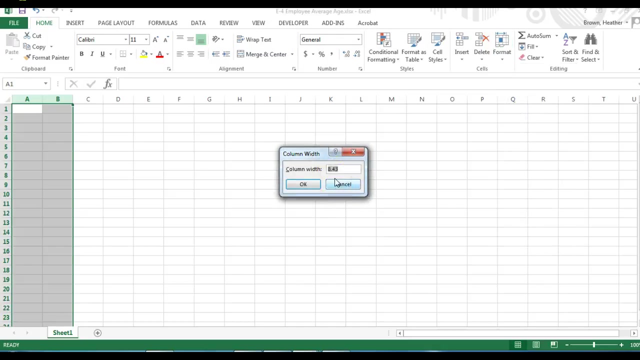 save as E-4 employee average age. Okay, so what we're going to begin with here is formatting the widths of the columns again, So A and B. we want to make those widths Home Format Column Width, both of them to 25.. 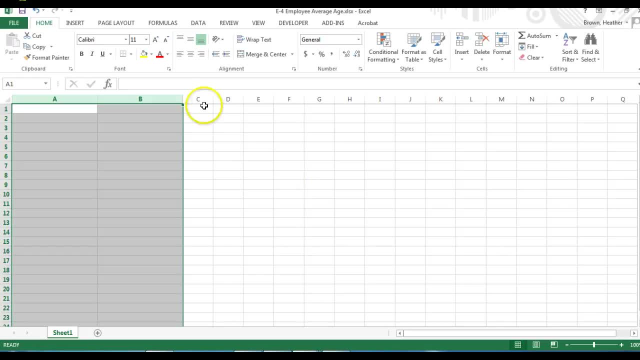 Click OK For column C. we're going to make that column width 15.. Then we're going to key in the data from E-4-1 into the spreadsheet And everything should be Arial 10 point, unless otherwise noted. So once again we're going to type in Arial. 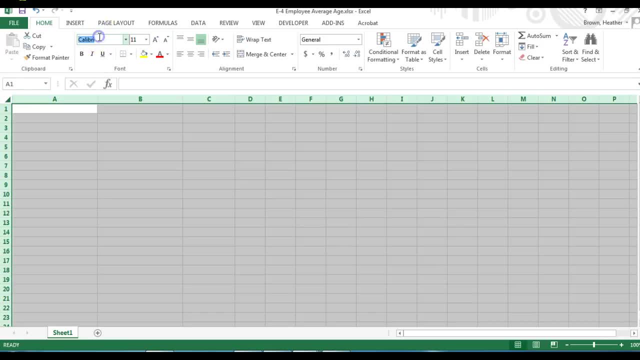 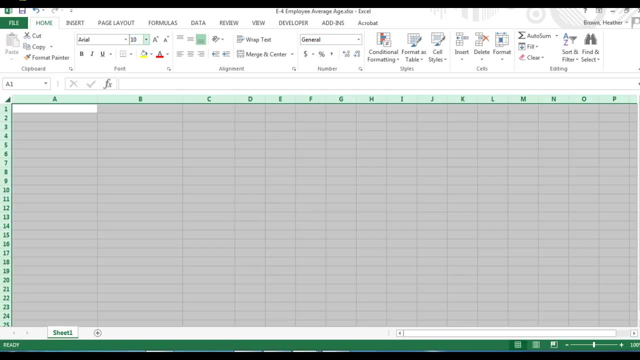 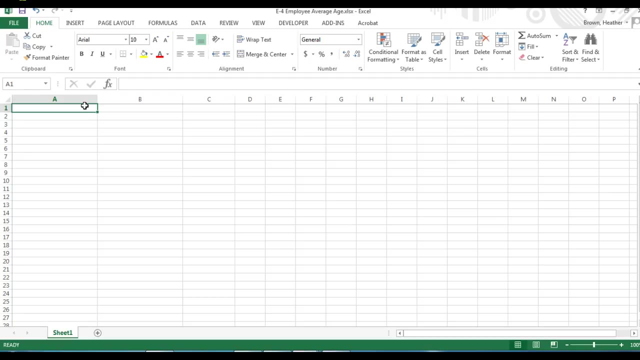 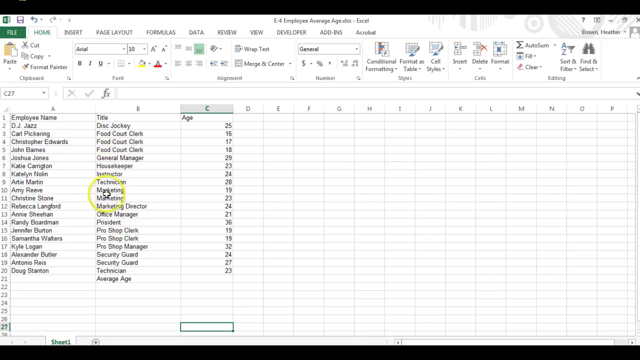 Whoops. first let's select the whole spreadsheet Arial, Enter And change this to 10.. Enter And then go to page 66 in your book and copy in the table. Okay, so we have everything typed in now And we're going to change the font size in cell A1 through C1 to 12 points. 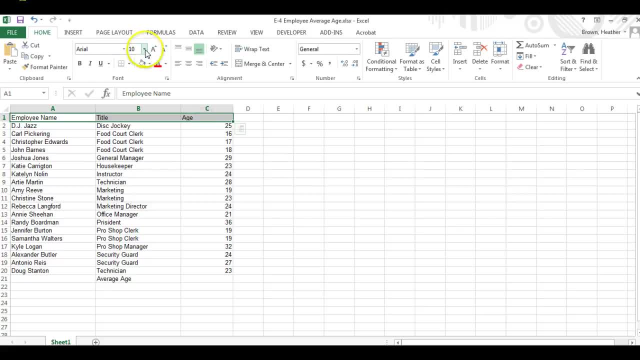 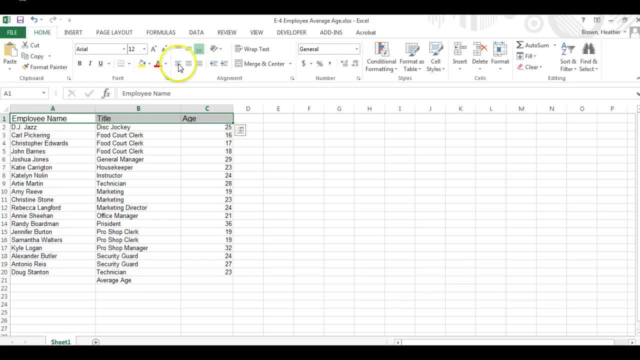 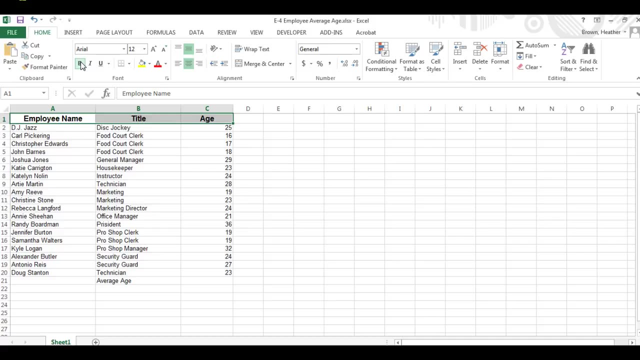 So we're going to highlight everything in A1 through C1.. I want to change that to 12.. We also want to center align the cells and bold them. Then we're also going to shade the cells A1 to C1 using a 25% gray fill color. 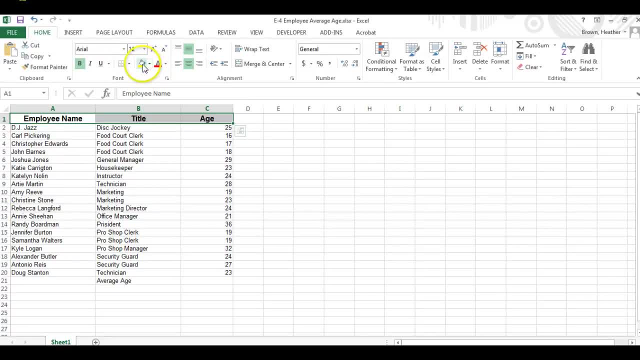 So we want to go over to fill And we're going to choose the 25% gray right there In the form. we're now going to enter a formula into C1.. We're now going to enter a formula into C21.. 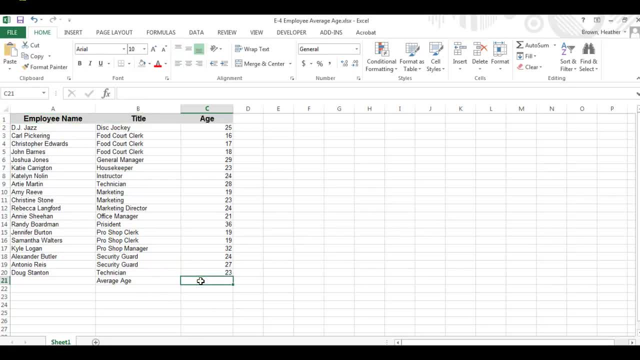 So we're going to go to C21.. And the way that you start entering a formula is always to hit an equal sign in Excel. So once we've hit the equal sign that tells Excel to start a formula, We want to do an average. 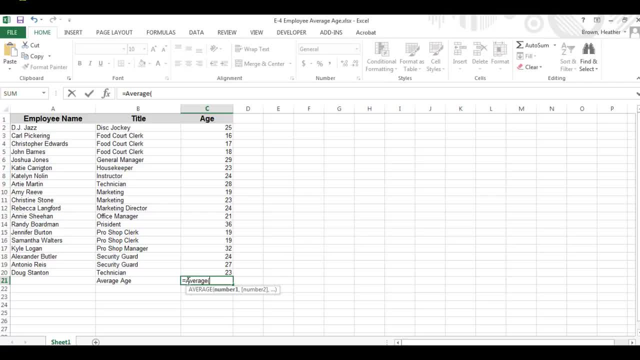 And you have to tell it which numbers to go through. So we're going to start with C2.. And we want it to go through C20.. Sorry, we're using a colon to say through Capital, C 20.. And see, it'll highlight the area. 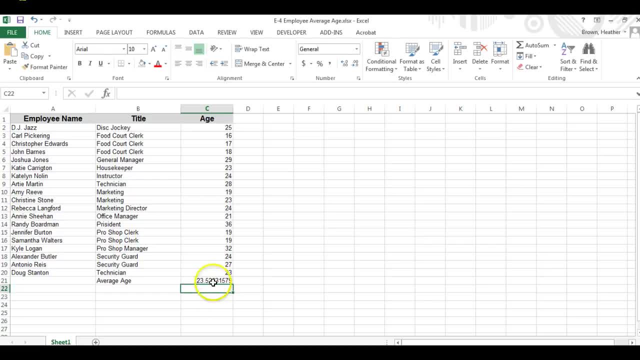 Close the parentheses and hit enter. Now we have an average. Okay, so C2 through 21.. We also want to make sure that they are center aligned And we want to tell it to have only two decimals displaying. So we're going to go over here. 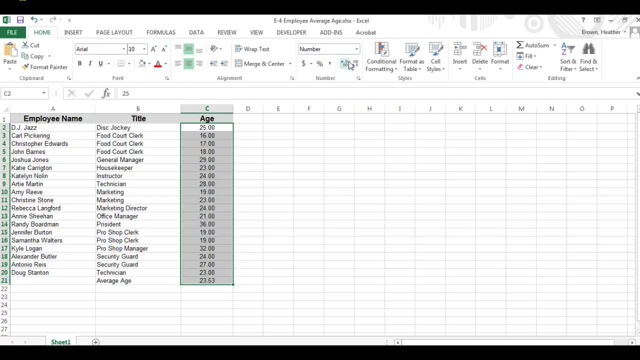 Increase the decimal to two. Then we move over to B21. And we want to make this right, align And bold. Format C21 also as bold. Create a custom header and key the text provided below as the header And center. align the header. 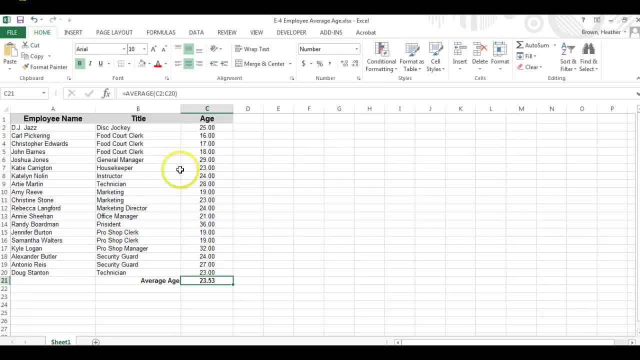 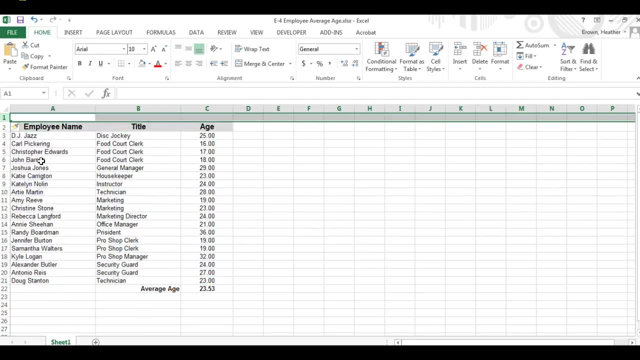 And set the font to Arial 14 bold. So we want to insert And we're going to select all three here And we're going to say merge and center And then type in the header: Skateboards Ink: Average age of employees.